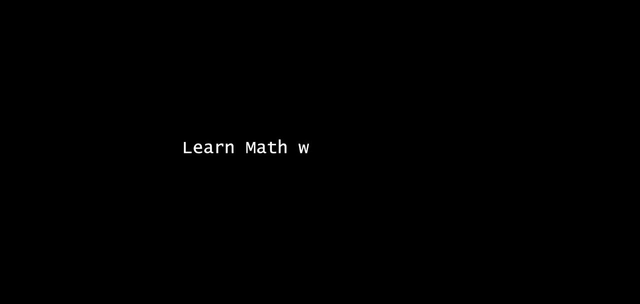 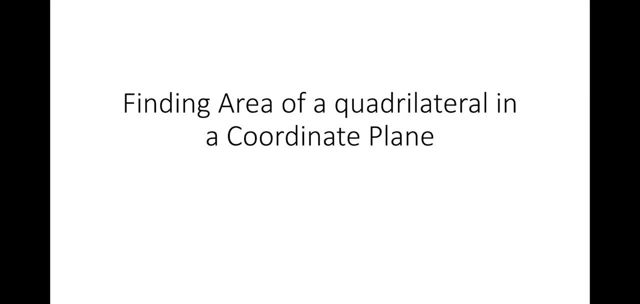 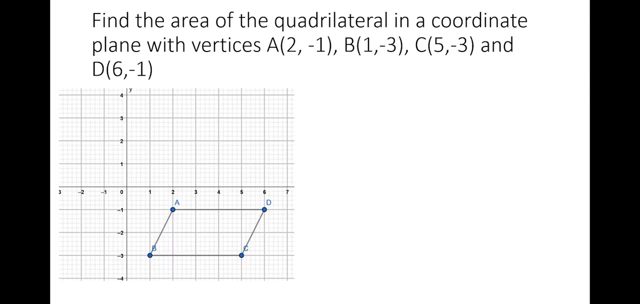 Find the area of a quadrilateral in a coordinate plane with vertices A is 2. next to the area of a quadrilateral in a coordinate plane with vertices A is 2.. Find the area of a quadrilateral in a coordinate plane with vertices A is 2. next to the area of a quadrilateral in a coordinate plane with vertices B is 2.. 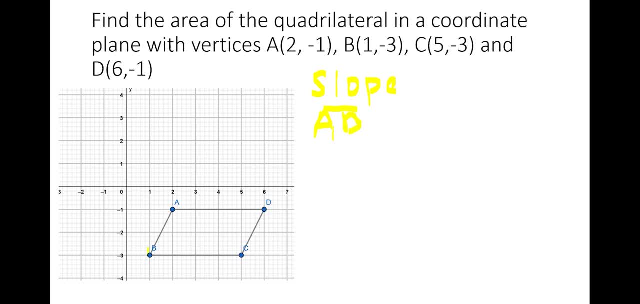 Find the area of a quadrilateral in a coordinate plane with vertices A is 2. next to the area of a quadrilateral in a coordinate plane with vertices B is 2.. Find the area of a quadrilateral in a coordinate plane with vertices A is 2. next to the area of a quadrilateral in a coordinate plane with vertices B is 2.. 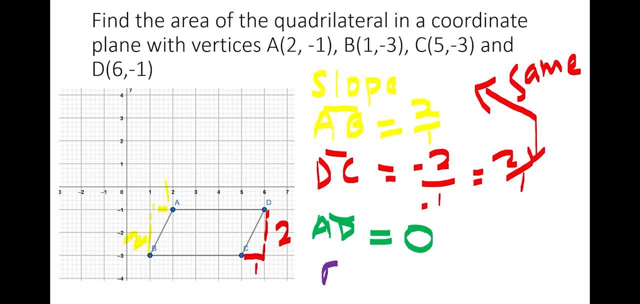 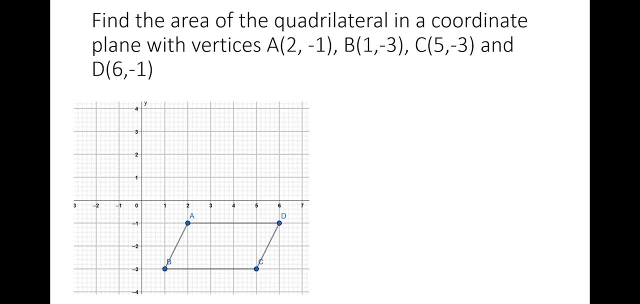 So find the length of each side side length. so AB we have going up to and write 1, we need to find C. so we know C squared equals A squared plus B squared. to find C we take square root of everything, so we have square root of 2 squared plus 1. 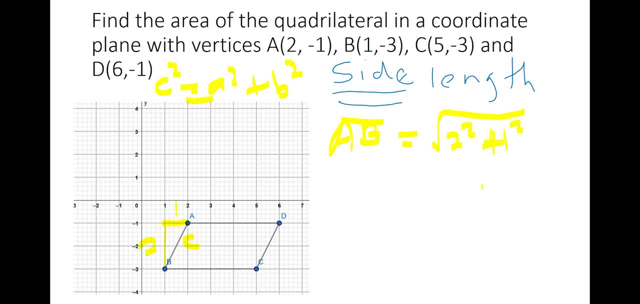 squared, 2 squared is 4 plus 1, squared is 5, so square root of 5, now we find the side 4.. DC, so 2 and 1,, 2 and 1, and this is our C, so it's 2 squared plus 1 squared, so it's. 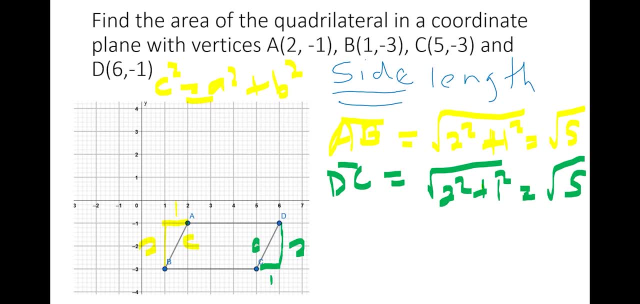 square root of 5. again now we want to find side AD. let's count our squares. since they are square units: 1 square unit- we can count how many squares are there between A to D, so 1,, 2, 3.. 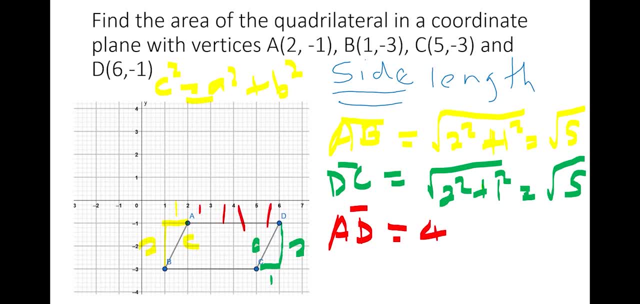 4, so it's 4 units. and then we find the side length for BC. it's not our squares 1, 2,, 3, 4, so it's 4, you can see these are same length and these two are same length. 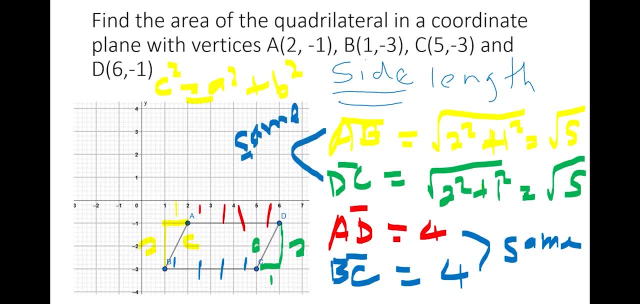 okay, So opposite sides are the same length. Okay, Okay, Okay, Okay. So opposite sides have same slopes and opposite sides have same length, So it's a parallelogram. to find the area of parallelogram, let's look at the formula. 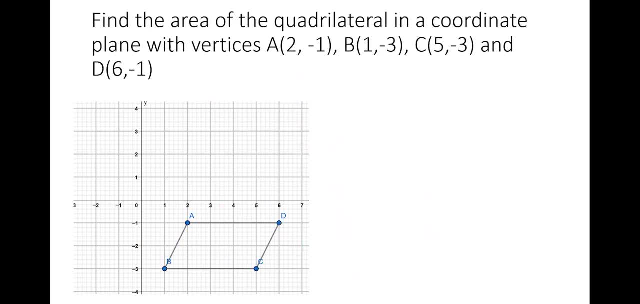 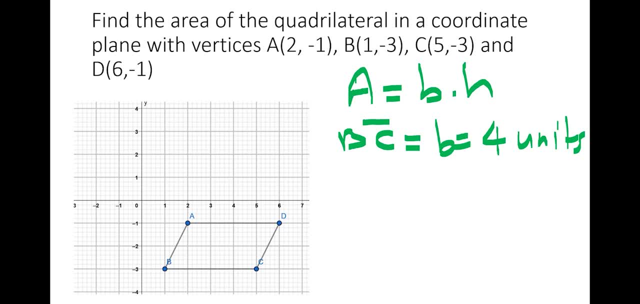 A and draw the line. So our height is 2 units, Point. you can say E, Point, Point, Point, Point A, E is our height, which is two units. Now we find the area. We find the area. 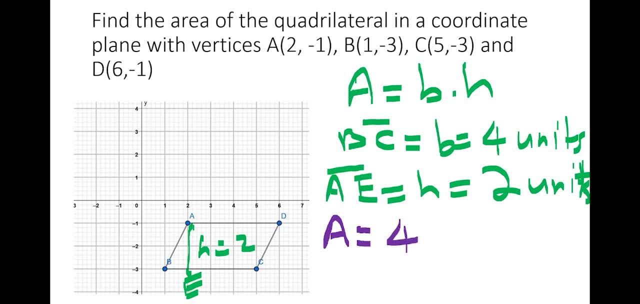 Object is 5.. 4. 15.. our height is 2, so our area is 8 square minutes. If I say it was a parallelogram, you don't have to prove it. but I said it's a quadrilateral. so what type is it? And then, after proving, 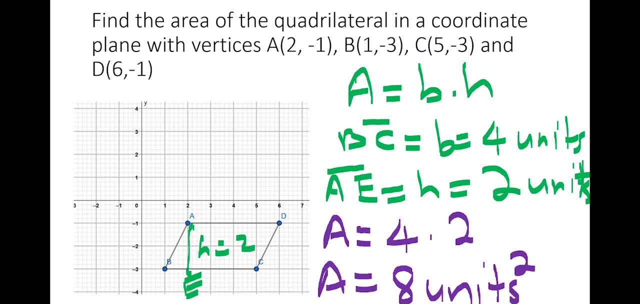 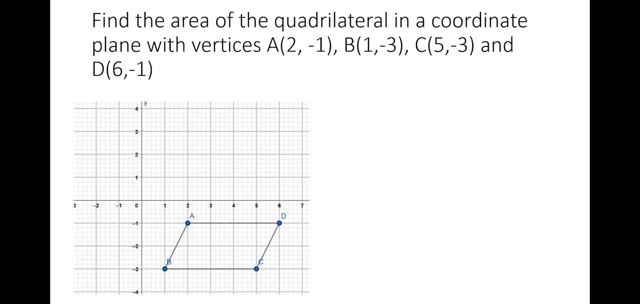 what type is it? then you use the formula for that type of quadrilateral. We can also find the area by breaking into different shapes. So if we break this into different shapes, I can see we have two triangles here and I see I have a rectangle. 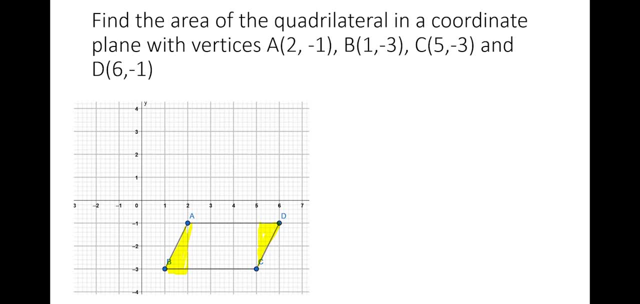 Rectangle is 3 by 2, so the area of the rectangle is base times height, which is 3 times 2, which is 6 square units. And then we see we have a triangle. both triangles are same. both triangles are same.